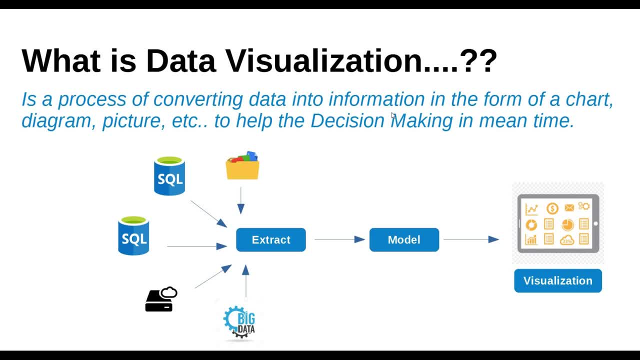 visualization is the raw data. what is stored in databases or data sources? we are taking it, we are converting it into the charts. so by seeing those charts, user must be able to make some sense or insights out of it and perform some actions. that is giving a positive impact to his business. okay. 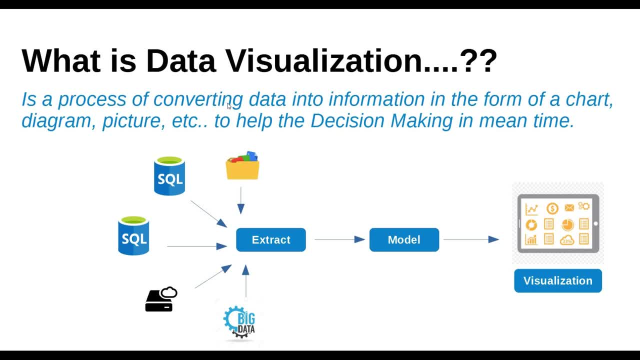 so that's it. we are basically converting the raw data into information in the form of charts and diagrams. okay, now let me move to the steps of data visualization. basically, there are three steps. includes those are extraction, model and visualization and, in extraction level, as everyone knows, extracting the data from data. 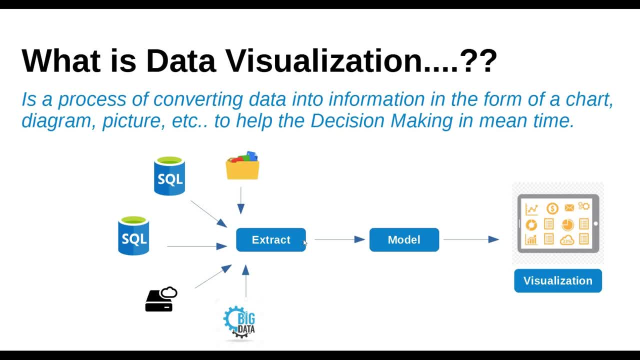 sources. the first part about bi tools are like. bi tools are compatible with any kind of data sources. let it be a big data data sources, let it be cloud based data sources, sql based data sources, or let it be flat file systems or excel files. so the first stage is extracting all the data from all these data. 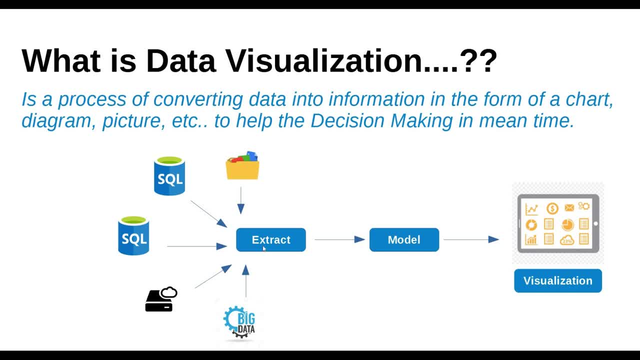 sources that is required for performing the creation of insights. and once the data is extracted, we will be storing it locally in the systems, so we could ensure the data availability all the time. okay, so once the data extraction process is completed, the data will be stored in stored in local systems. after that, the stored data will be passed into the model. so what is happening? 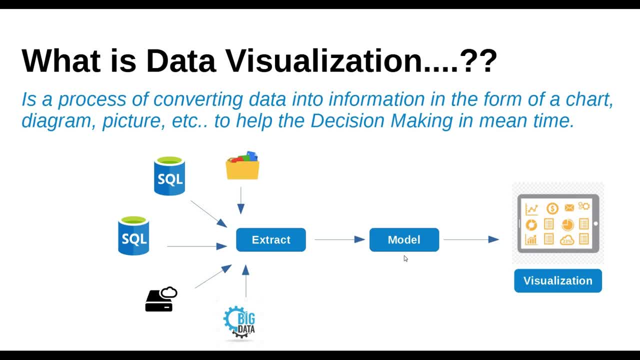 is basically the data cleanup part and that making the in model. what we are exactly doing is this raw data. we are cleaning it up first and making it most compactable for the visualization. so model part is very important because an inefficient model could give performance issues in the visualization layer. okay, so what is happening in model is we 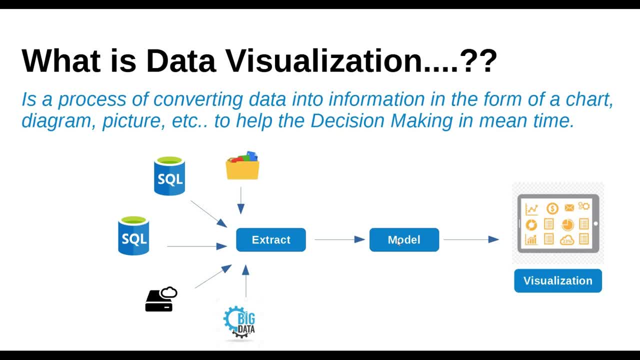 are taking the data. we'll perform the cleanup operations like handling null values, removing unwanted columns and rows and creating the interlink between tables and creating the calendar for time series operations. all those things will be done in model layer. okay, the outcome of model layer might be a single table or a set of tables those are interlinked. okay then. 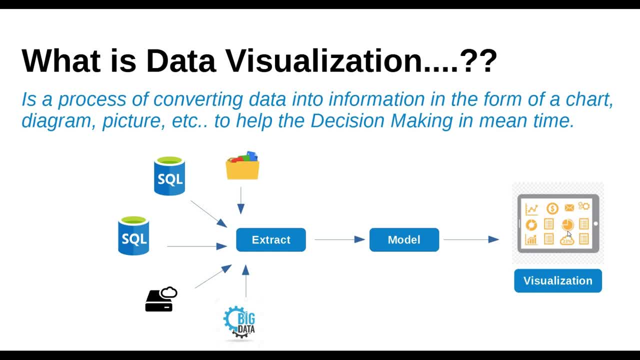 comes the next layer, that is, visualization. in visualization, what we are doing basically is we are creating charts out of the result of this model. so this model will, as i told you, the model will be giving you a table or a set of table. those are interlinked. now we'll create charts out of it. 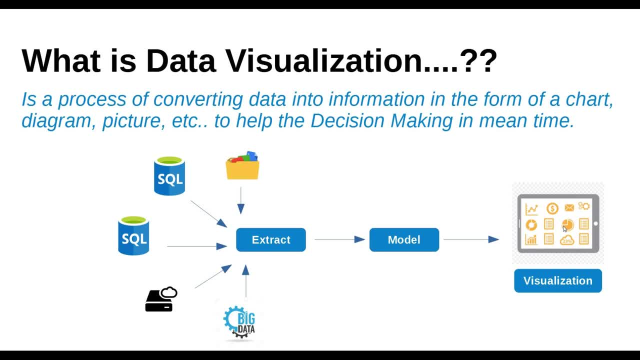 so basically, most of the charts required a dimension as well as a metric. so dimension is nothing but the columns, that is, the that is coming out of the uh model layer and matrix is nothing but the operations that you are performing on that. those columns aggregate operations. so 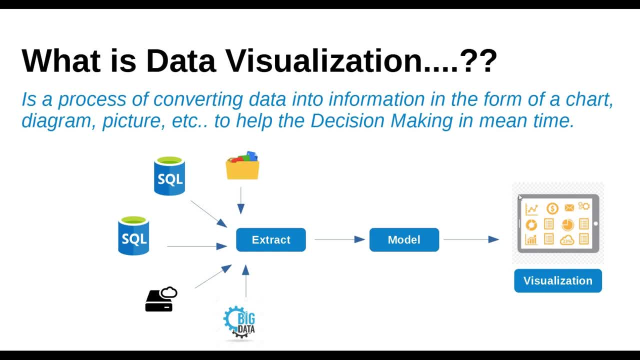 aggregate operations include count, sum, average, standard deviation. all those things are the basic metrics that we are performing on on top of some columns that is coming out of model layer. so understand only this. much about data visualization. now we will be moving into the importance of data visualization. 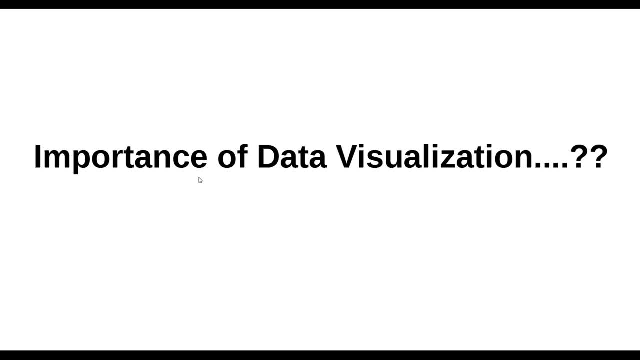 importance of data visualization. so here we will be discussing how important is to visualize the data to get the insights out of it. so if you ask me a question, is it necessary to visualize the data to understand the data? so i would. i would say no, it's not always necessary to visualize to understand. 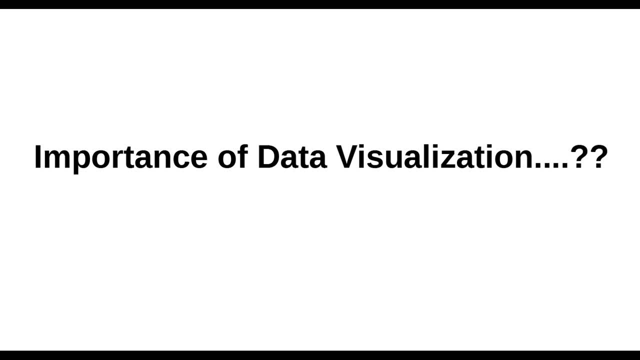 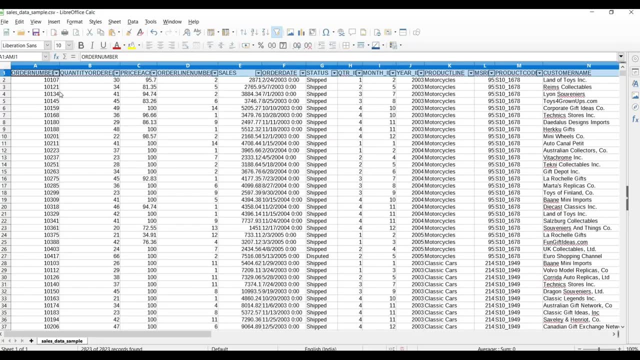 what is the advantage that we are getting if you are visualizing it? that i'll try to show you here. so let's say i have my data in a simple tabular form. i have downloaded one data set from kaggle, so this data set basically tells you the genes. so you here, you can see all the properties of data. 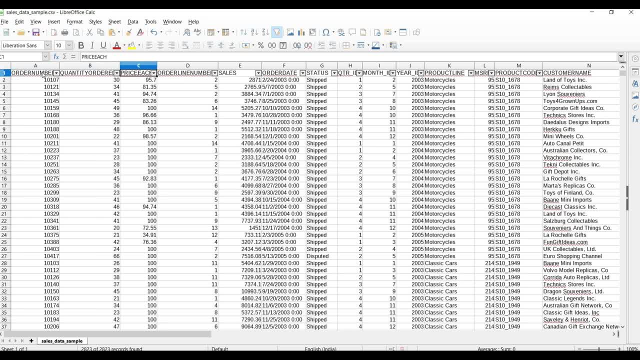 sales transactions like order number, quantity, order price, each sales amount, order date, status of the sales, all those things you can see here. so let me try to analyze it, analyze it and get some insights out of it. okay, so i want to know what is overall overall amount of sales that i have. 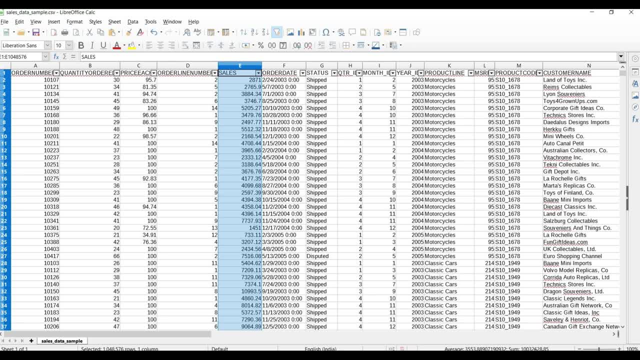 performed. i can just select that particular column and get you know. okay, it's around 1 crore 32 000 and i want to know what are the overall sales transactions has happened so far so i can select this order number column and take a distinct count of it. so it will be like around uh 1 lakh 48 000. 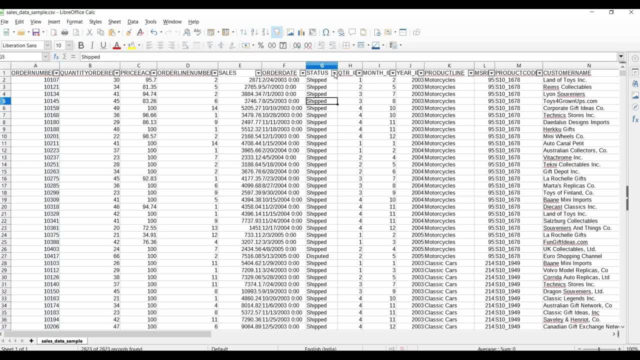 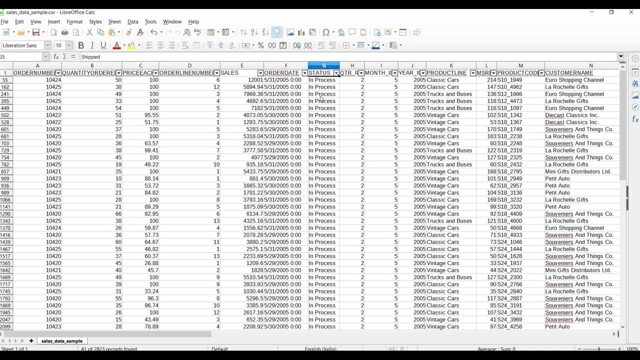 and i want to know what is the current status statuses of my transactions. you can select it here. status are available. so i want to know what is the in progress sales transactions here, so i can select in progress. so i'll get the. i'll fit. i filtered the data based on that in progress status. 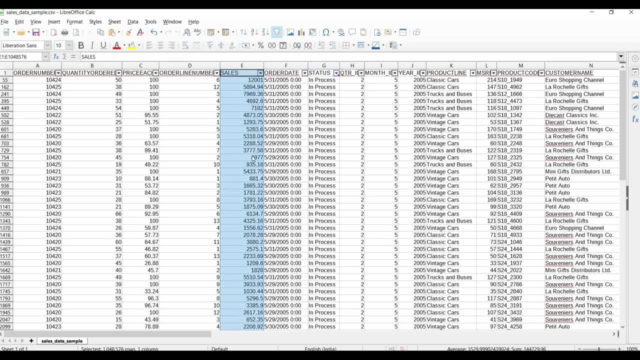 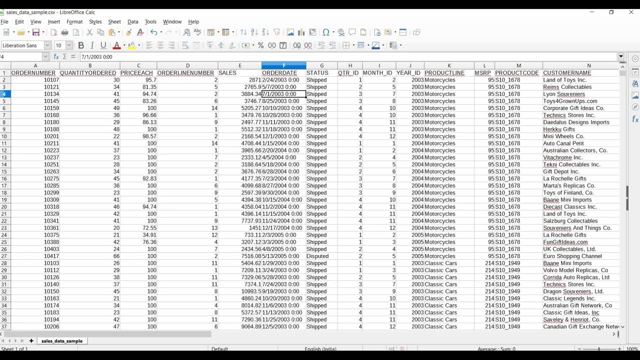 so here i can get the in progress sales amount. it's around 1 lakh 44 000.. see, i can analyze this data without visualizing it also, but what is the advantage if you are visualizing it? that's what exactly the question here is. so i have created a dashboard based on this data in click sense. 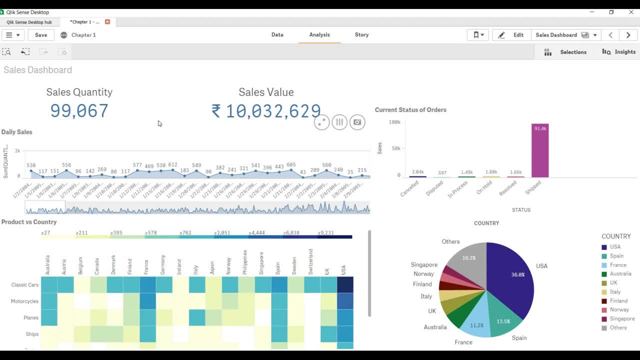 so here is my dashboard. it's a simple dashboard. there is no much visualizations included, so it is just to showcase what is the importance of visualizing the data. so here i have created a matrix: sales quantity. so sales quantity is nothing but the sum of ordered quantity. how many? 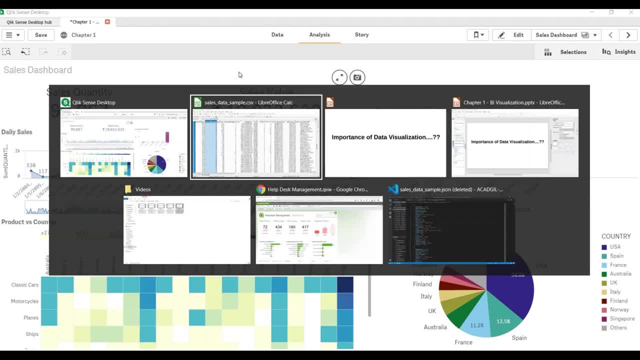 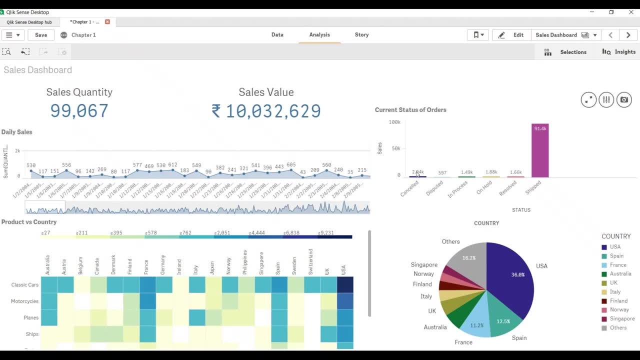 number of products that i have sold and sales value. sales value is nothing but the sum of sales. here what's the worth of sales that i have done, and here you can see the current status of the sales orders. and here you can get a time series trend of sales and you can see the. 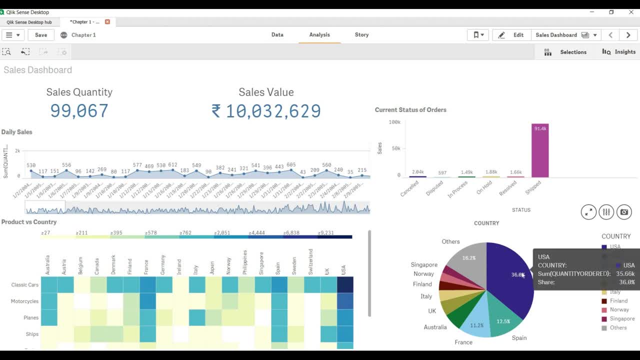 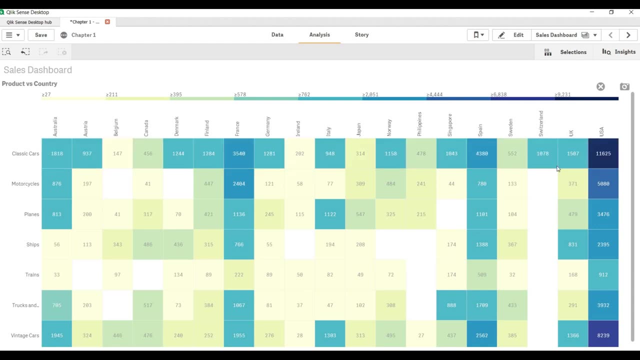 country, wise sales. so here you can get an okay in which country you are making- usa making most of the sales, and the second one is spain, third one is france, so on it goes on. then here there is a map, heat map for country and the product. so here you can get to know in usa i'm selling classic cars. 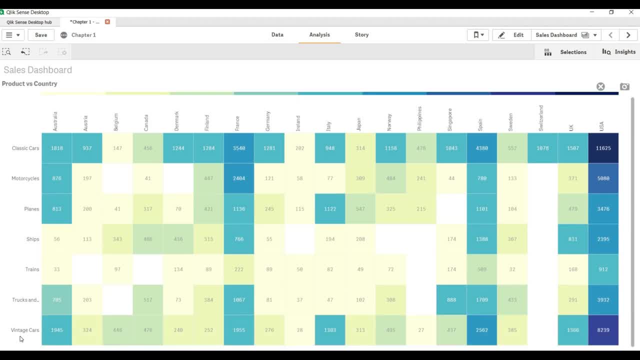 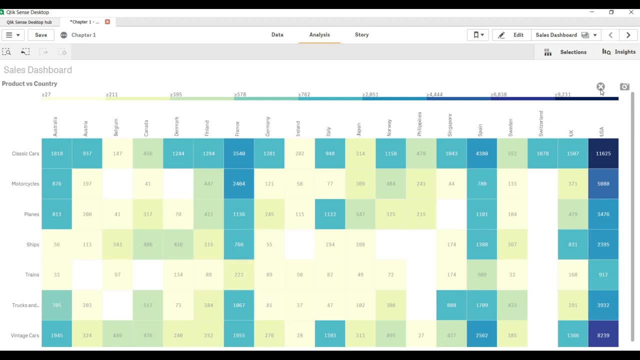 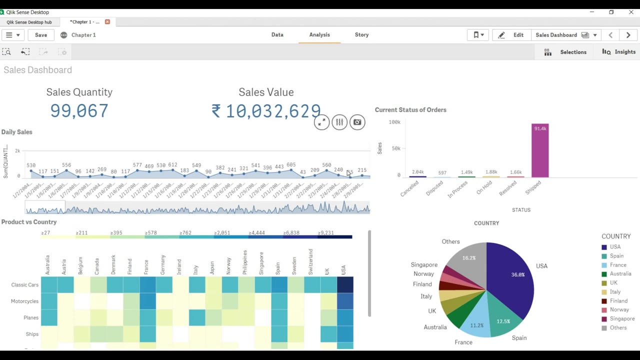 and vintage cars. second, second, second one is vintage cars. motorcycles is also very high. most of the sales are happening in usa. so those kind of insights you can make. so if you compare a tabular form and a visualized form, i'm getting them. i'm getting more insights in 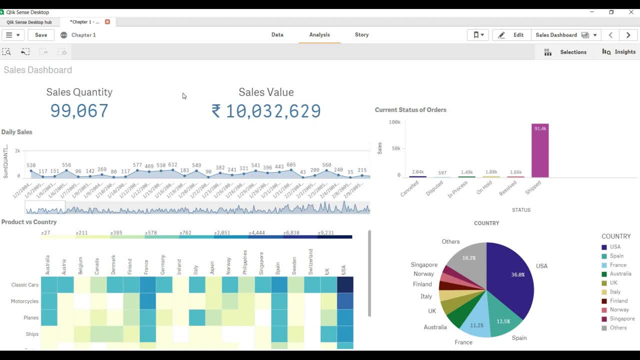 mean time from a visualized form. so in business it is very important to get the get to know the data as soon as possible so they can perform the actions. they can more focus on the actions to be taken instead of spending more time on analyzing the excels or writing sql queries. 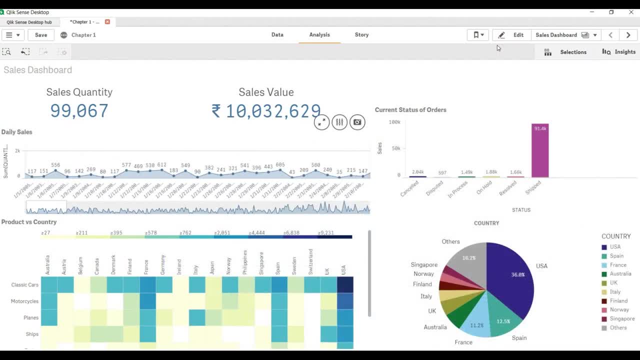 to get to know the information. so, see, and one more advantage here is: see, you can make any selections and you can get to the data. suppose i just need to know only sales that i have done in us, you can just select us. so the whole dashboard is getting changed accordingly. see, this is overall sales.